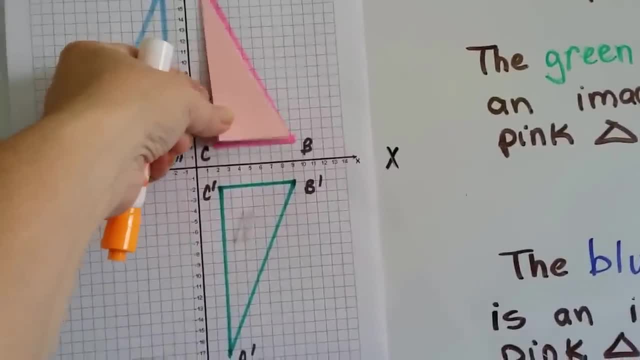 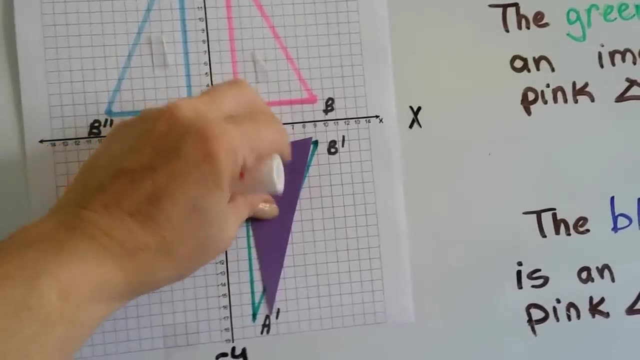 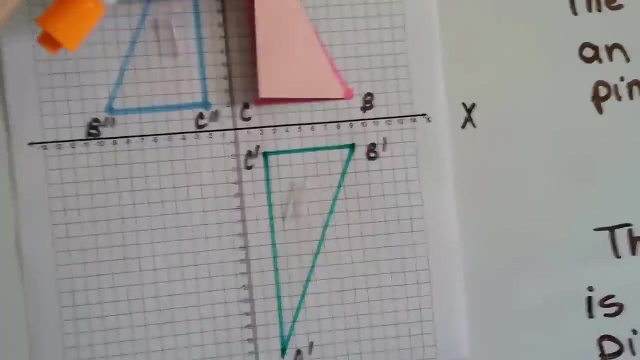 pink triangle and the green triangle is the reflection of it. see that we can just go like this and it'll flip and be the exact same shape. we can even do it with the blue one. we can take the pink triangle and we can flip it and it'll. 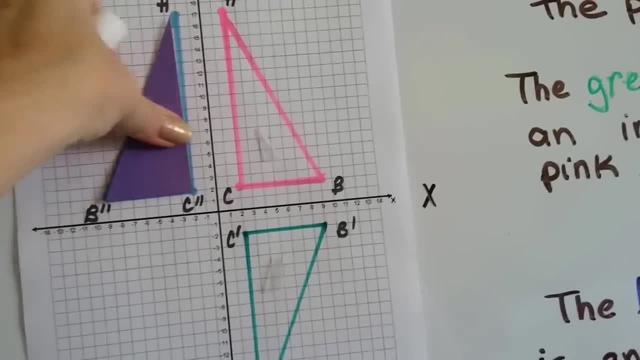 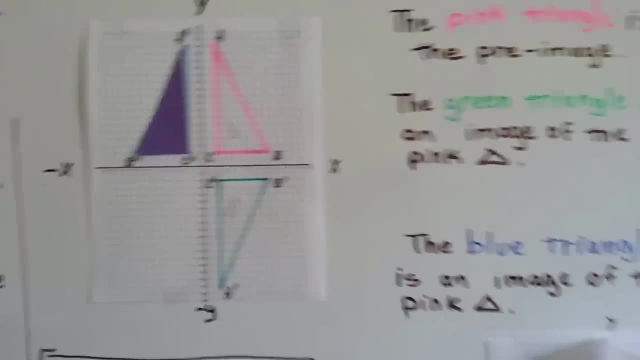 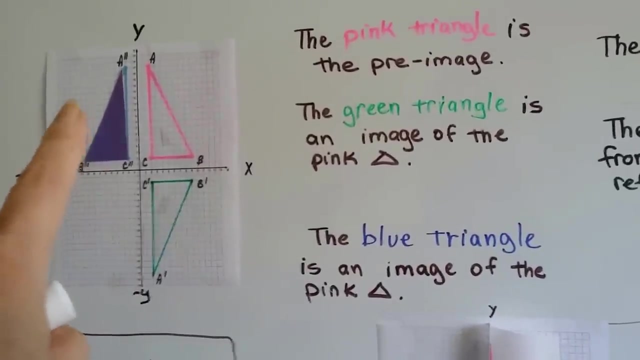 lay perfectly here. see, it's hard to do it with one hand and I have a bad arm, unfortunately. this is the reflection, ok, so the pink triangle is the pre-image, the green triangle is the image of the reflection and the blue triangle is also the image, the reflection of the pink one. see, and I've got them labeled. see that this is. 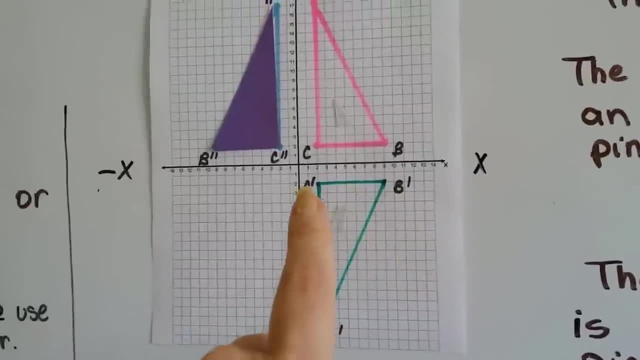 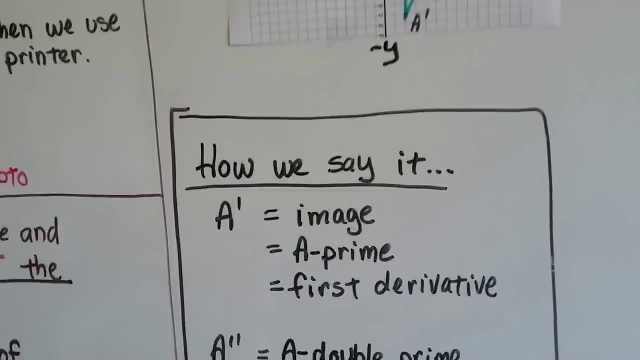 ABC and this is triangle: a prime B, prime, C, prime. and the way you would read this is a double prime B, double prime C, double prime. that's what those tick marks are. that's how we say it. that's a little tick mark, it's not a one, and 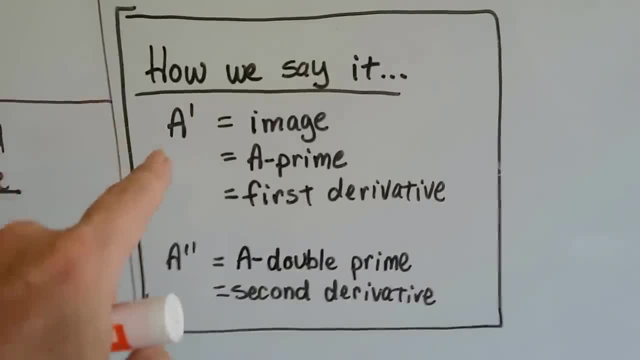 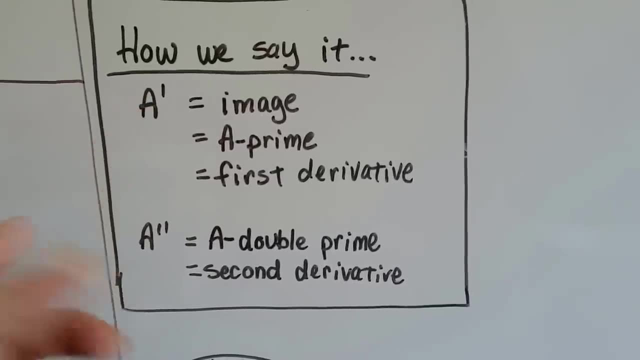 it's not eleven, it's a little tick mark. ok, it's like a teardrop and the way you would say it is a prime. it's the image. it's also the first derivative. we talked about derivative a couple videos ago. when you see two of these lines, that's 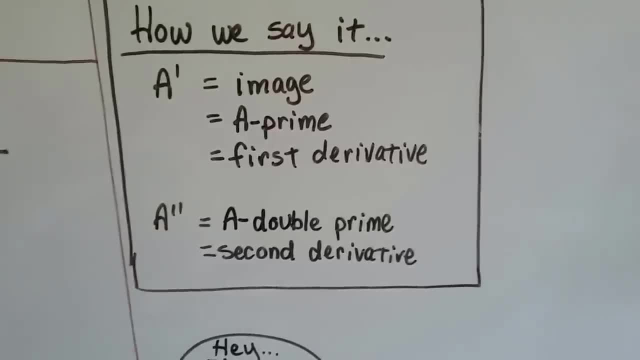 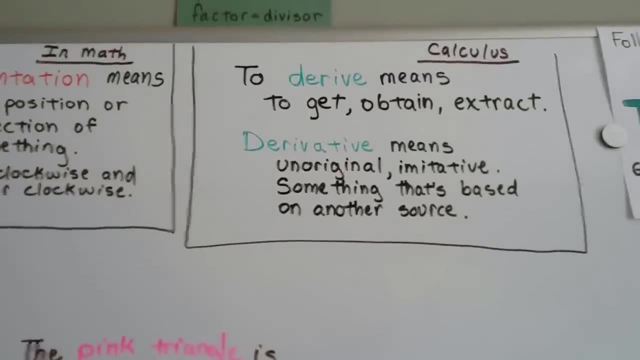 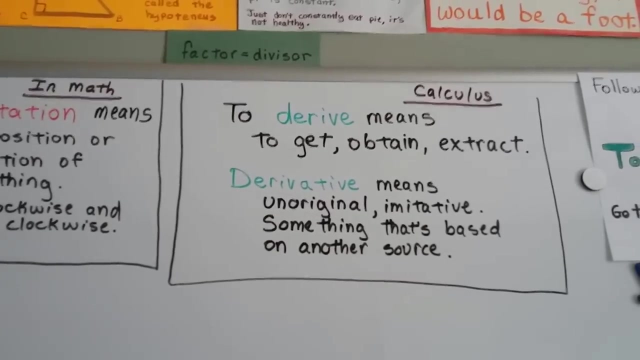 referred to as a double prime. it's the second derivative. ok, and to derive means to get something, to obtain something, to extract it. so derivative is something that's unoriginal, it's not original imitative it's an imitation, it's something that's based on another source. 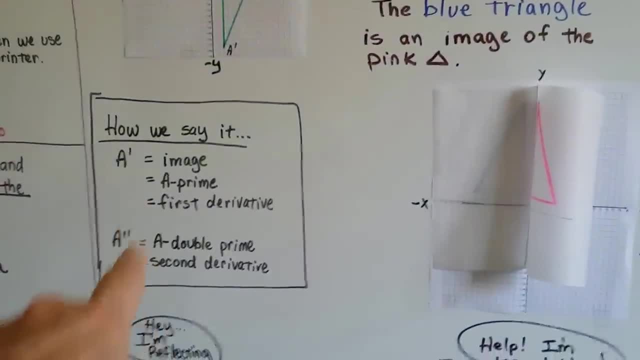 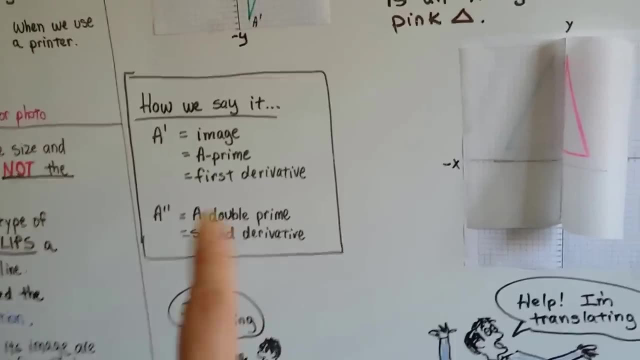 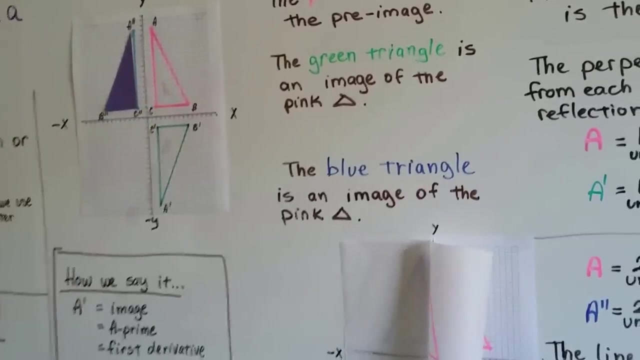 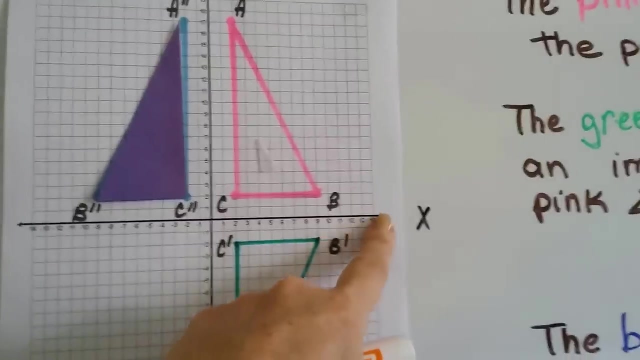 ok. so the way we say this with the little tick marks is prime and double prime and I, if you saw three, what you think it would be called. so this is a reflection and the green one is a reflection. see that now? the line of reflection for the green triangle is the x-axis. do you see this? here's the x-axis. 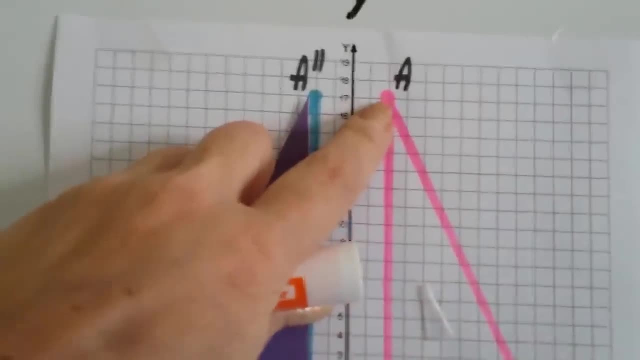 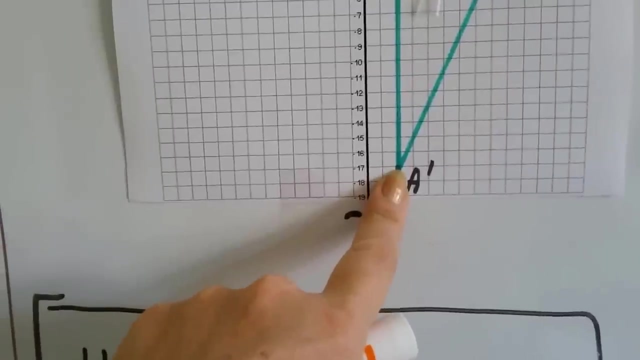 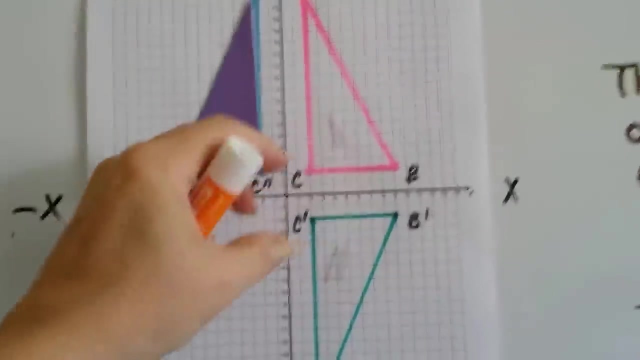 axis and if you look, A is at 17 up here on the Y and it's at negative 17.. See that. So it's the same distance from the X axis here as it is here, And look, C is two squares. 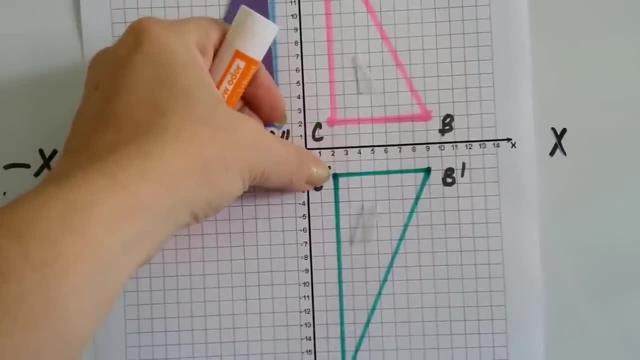 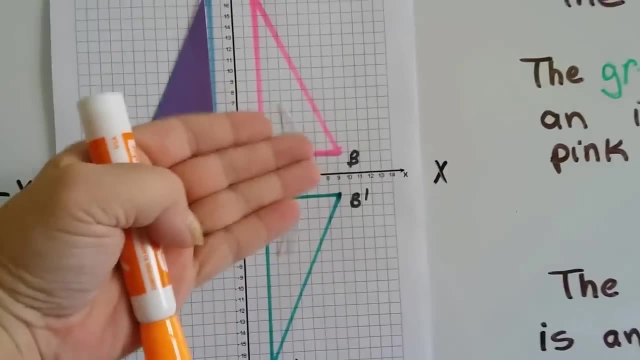 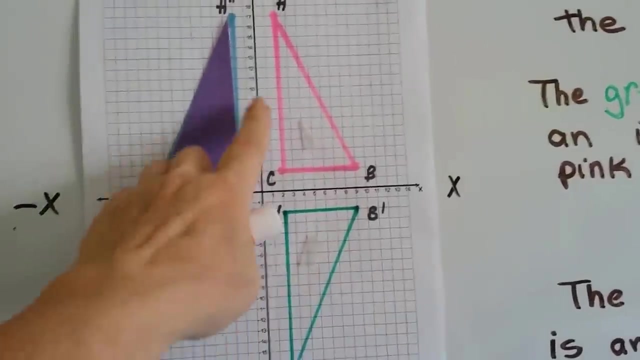 away from the X axis and C prime is two squares away from the X axis And B is two squares away and B prime is two squares away. See that. It's exactly the same distance across this line of reflection for both of them. See that, And this is two squares away, and 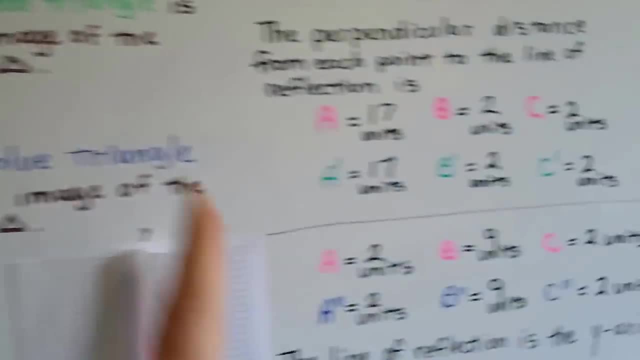 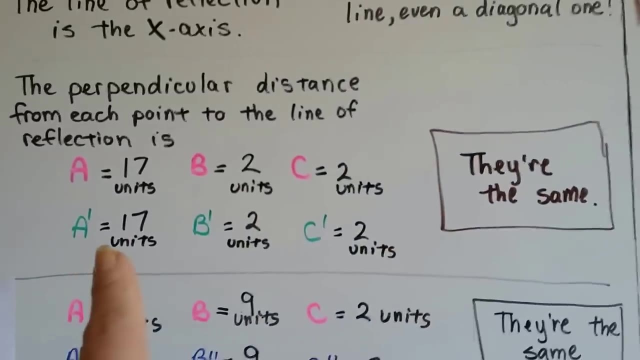 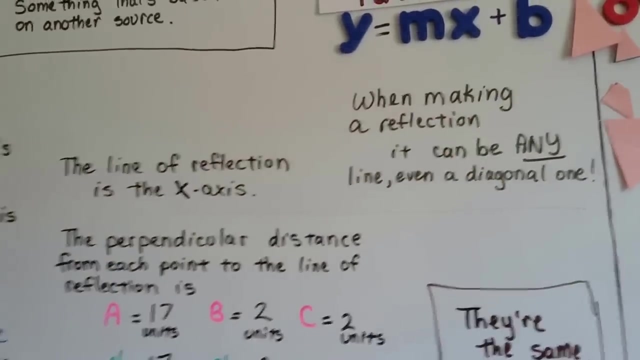 this is two squares away for this one. See that. So the perpendicular distance from each point to the line of reflection is the same. They've got the same number of units. Now, when making a reflection, it can be any line, even a square. 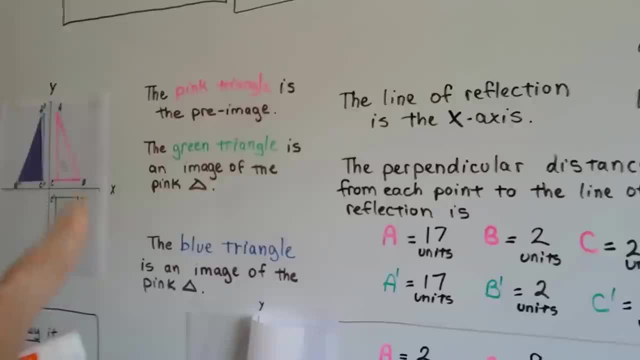 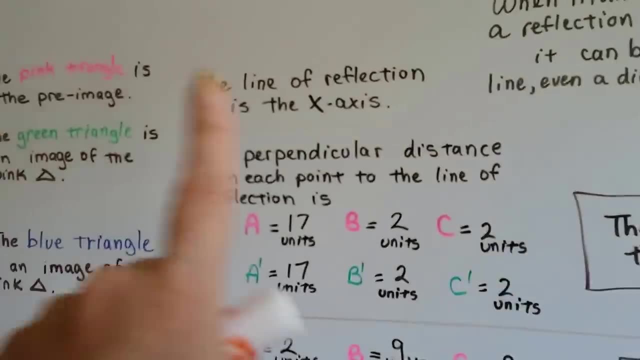 even a diagonal one, even one of these lighter colored lines on the grid. It doesn't have to be the X or Y axis, It could be any line, okay, But we're just using the X and Y axis now to make it easy for you all, right. 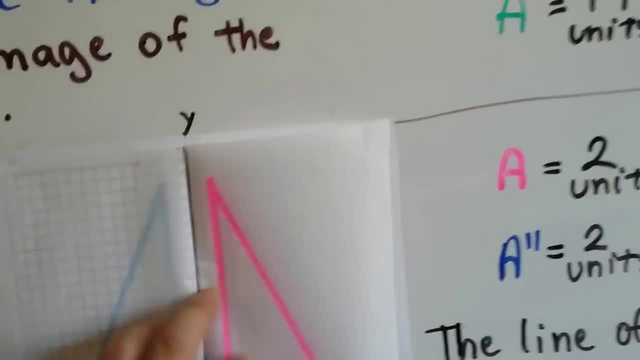 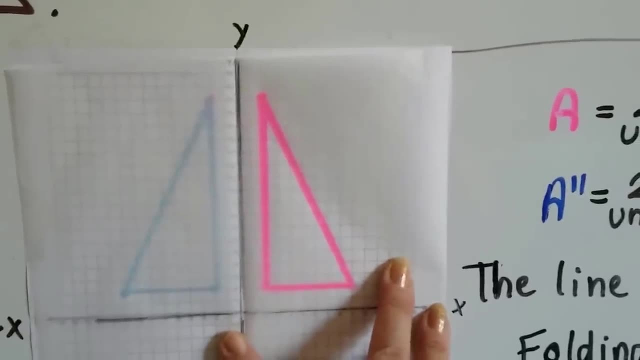 So now let's look at this blue triangle. Look what I did here. I made some tracing paper and I put this pink triangle there And when you lay the tracing paper down you can see it perfectly. See that? And then I drew the triangle on the tracing paper. Now here's. 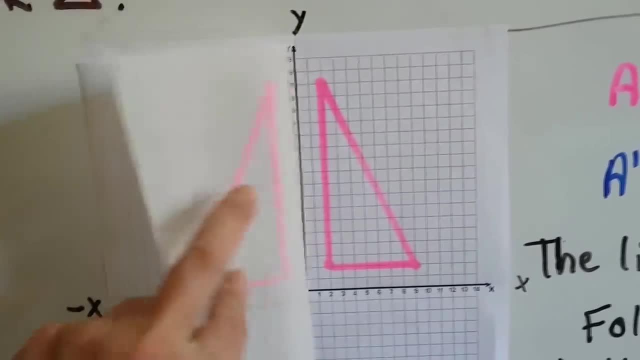 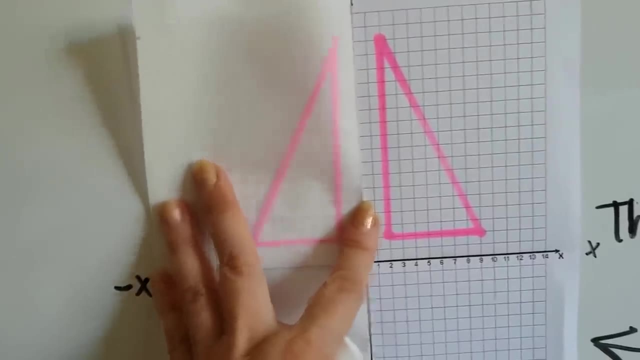 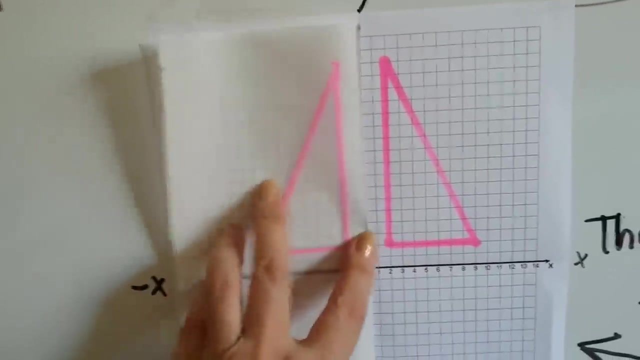 the blue triangle underneath it. and when I flip the tracing paper over, folded right along the Y axis, it lines up perfectly with the blue one. See, Can you see the blue one underneath there? But when I fold it on the Y axis, which is the line of reflection, it 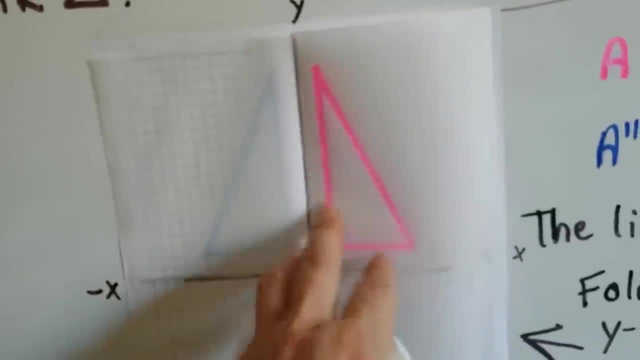 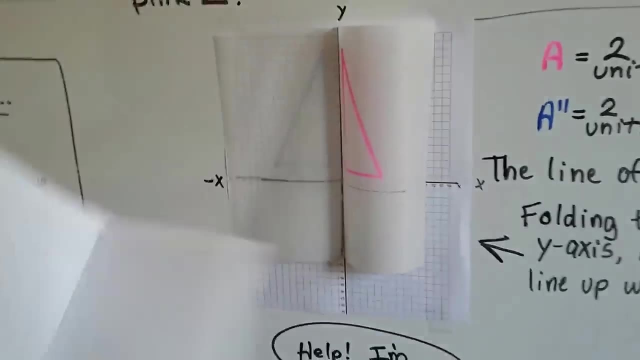 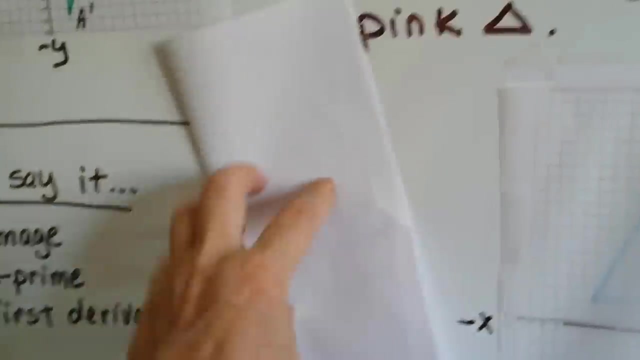 lands on it perfectly. See that If I were to get a piece of graph paper and I had triangles paper and I had triangles drawn in every quadrant, I would be able to take the graph paper, fold it in half and line up the triangles on this quadrant, on these.